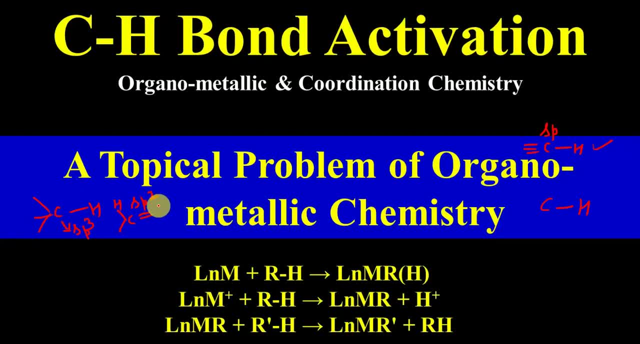 So breaking this bond in alkenes is difficult as compared to alkenes And the easiest way is to cleave this bond. in case of alkenes Means sp3, hybridized carbon atom. So CH bond of any alkyl group can be cleaved, but it needs some catalyst. 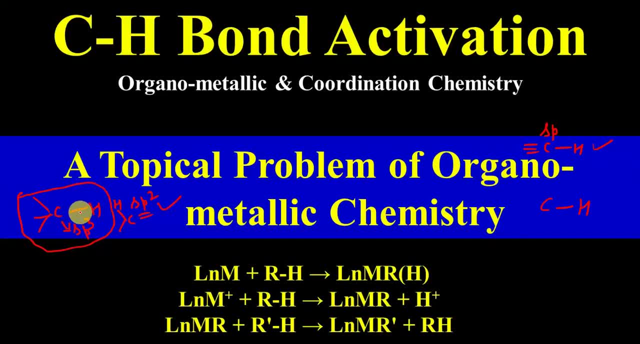 And there are many organometallic compounds, transition metal compounds, which act as efficient catalyst for the cleavage of this. Now, why we need the cleavage of this bond? Because if we can activate or functionalize this CH bond, it will be very beneficial to synthesize a large number of organic compounds. 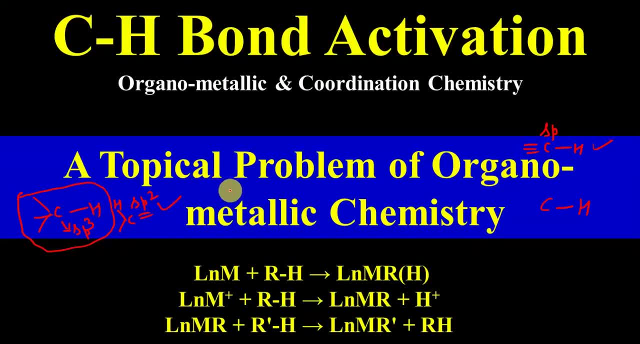 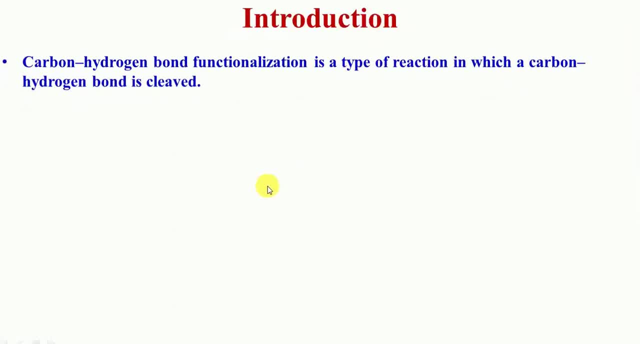 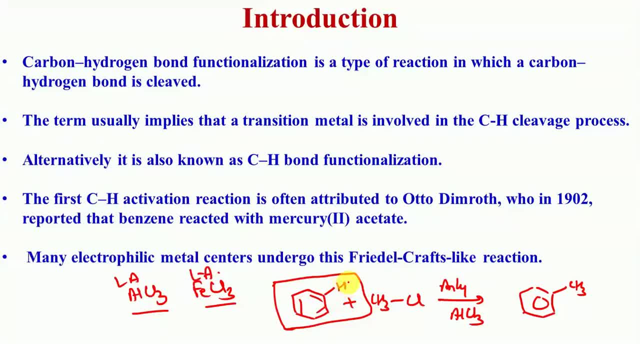 H is coming out and in its place methyl group is joining In Friedel-Craft acylation. acyl group is joined here, So this CH bond is cleaved. Joseph Chet observed the addition of CH bond of naphthalene by ruthenium zero complexes. 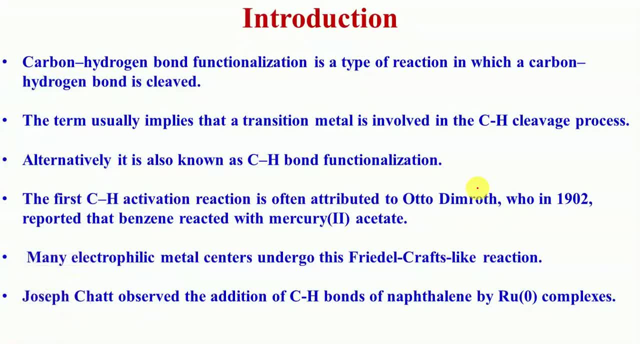 also So naphthalene is similar to benzene. What is the difference in structure? That benzene has only one ring, but naphthalene has two rings, Two fused benzene rings. The CH bond of this was added oxidatively to Ruthenium Zero complexes by Joseph Chet. 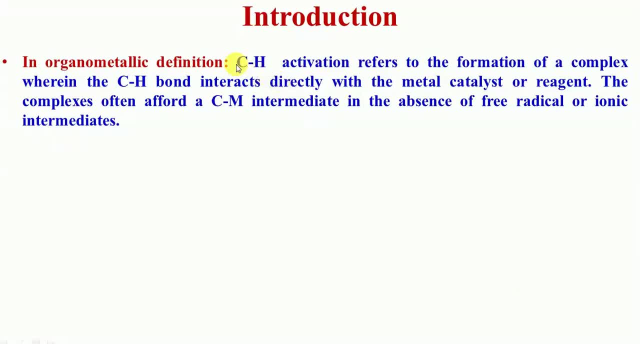 In organ metallic chemistry. what is its definition? So CH bond activation refers to the formation of complex where in the CH bond interacts directly with metal, catalyst or reagent. So let, this is a metal in which the metal has oxidation state plus n If it reacts. 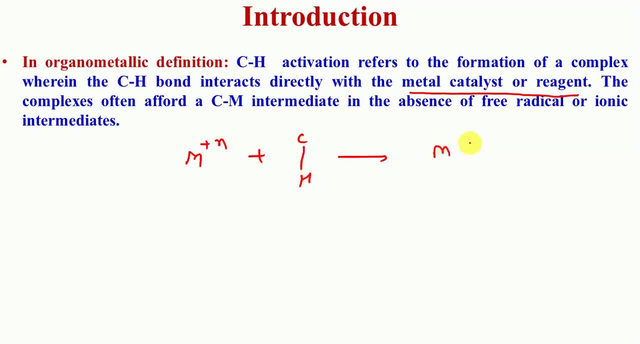 CH group say we will get MC and H, so metal alkyl or metal aryl complex and a metal bond here. in addition, metal oxidation state by two units will increase. so in this case, what is happening with this metal center in which more ligand present can be present? what is coordinating with it? what is joining? 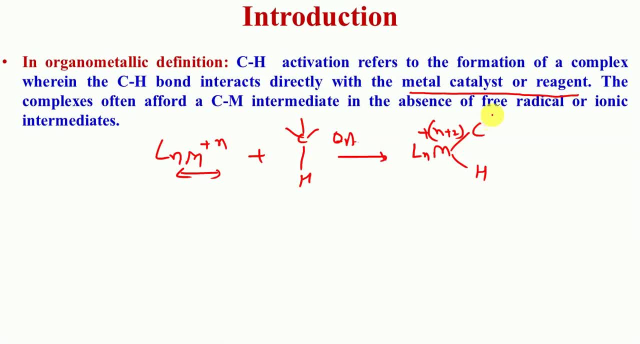 this CH bond is undergoing cleavage and oxidative addition is happening here. so what we are getting? we are getting metal carbon bond and metal hydrogen bond product is being made. the CH bond activation is frequently used as an organometallic term to describe certain metal mediated. 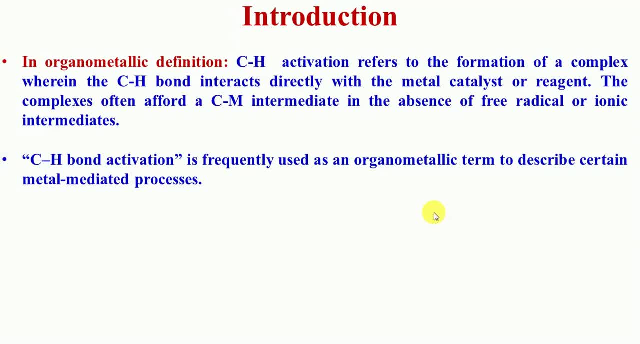 processes, many reactions. we have studied that, for example, alkene, hydrogenation, alkene isomerization. in all of them also CH bond activation was done. for example- you will remember this metal was metal along with you here- beta- hydride elimination, etc. We have been studying these reactions. so It, carbon atom, with which the metal is connected. 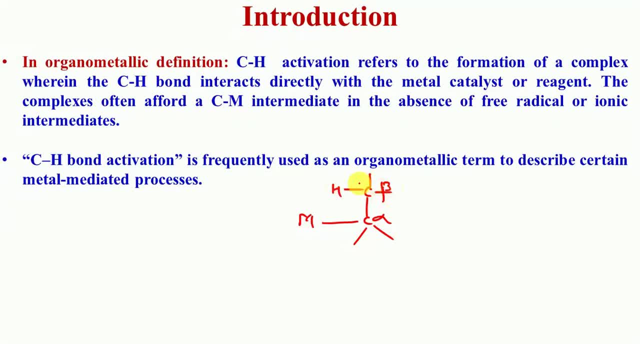 alpha be a beta. here is beta on which the hydrogen atom along with beta carbon, This done, accompagnant acoustic hydrogen with metal and also become along with metal, with hydrogen bond, along with Alcane formation, wasよね. so hello, basically the cleavage of this someone. she also example is a state of activatonch bond. 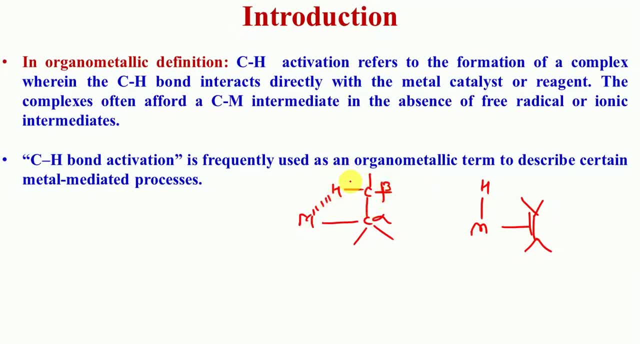 This is also an example of CH bond activation in which we were talking about beta hydride elimination. So another example of this CH bond activation is beta hydride elimination And in which reaction we have observed. We have observed this reaction in alkane hydrogenation and alkane isomerization. 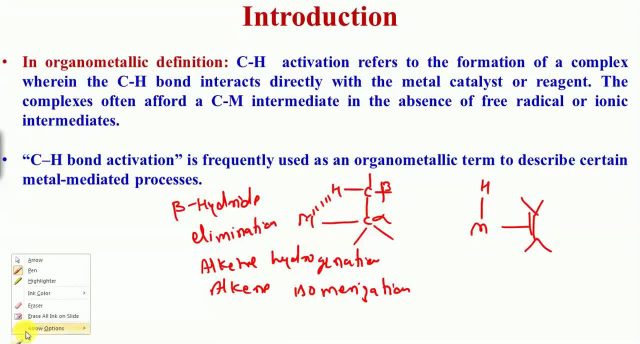 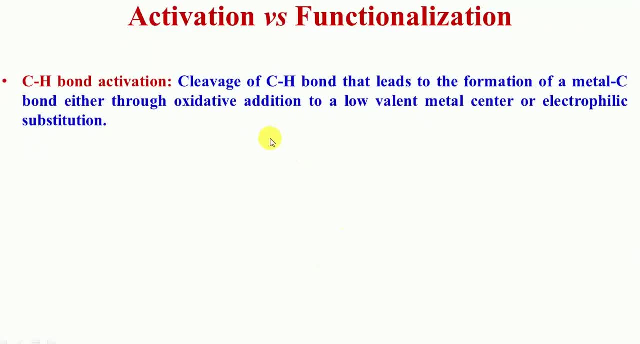 So in these reactions we have discussed these things already. So what is the difference between activation and functionalization? So activation is simple. The cleavage of this CH bond, The cleavage of this CH bond, of any alkyl or aryl group, this bond will break and it will connect with the center of the metal. 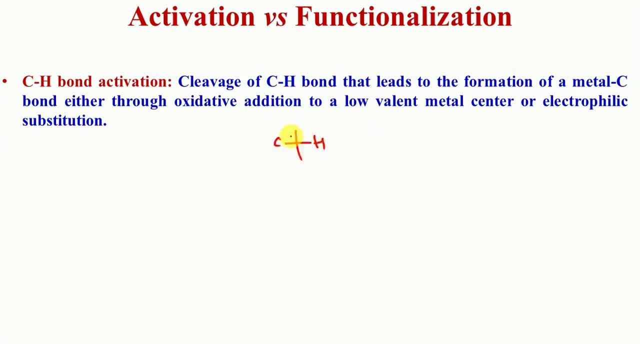 That is called CH bond activation. Activation means we are increasing the energy of this bond and breaking it, Because when the energy is more it will be very easy to break. it Means we are making it unstable. And when we talk about CH bond functionalization, then what is in it? 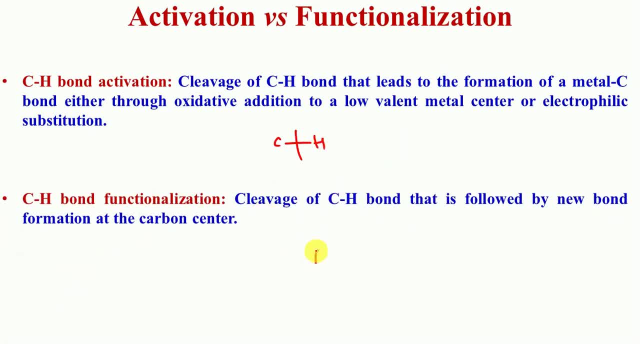 When this bond is cleaved then it will have some other functional group, with carbon For example, if the oxidative addition of this bond with metal is done here. after that any group, any X group, will be attached to this metal. carbon and carbon will be attached to this group. 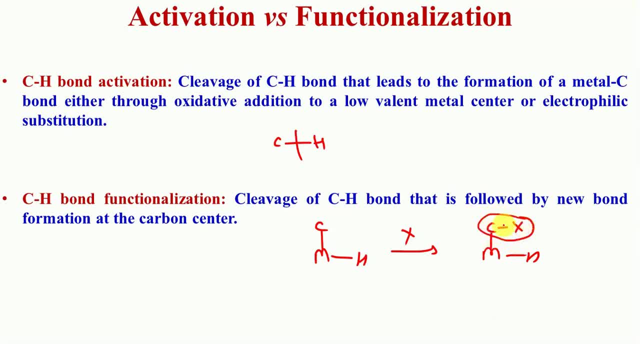 So this is basically functionalization. So we have added a new group with carbon. This is referred to as CH bond functionalization, in which we have functionalized the carbon in a way that we are removing the H and adding a functional group to it. 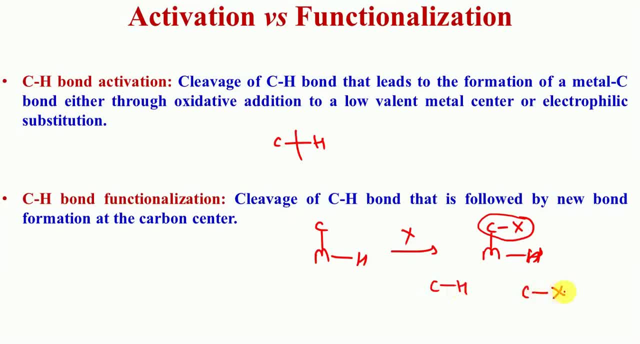 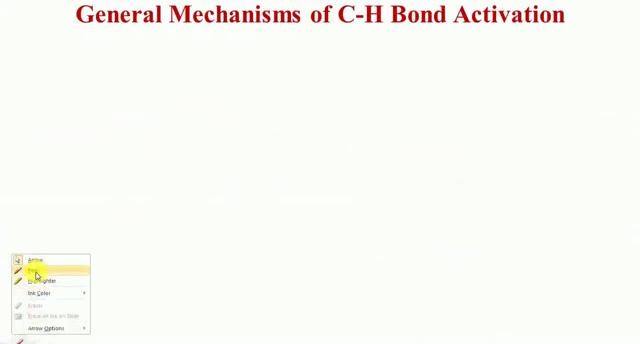 So first it was CH bond and now it has become CX bond. So this is functionalization. This is functionalization and this is CH bond activation, in which the simple cleavage of carbon and hydrogen bond is taking place. Now there are basically five ways, five types of mechanism from which CH bond activation can be done. 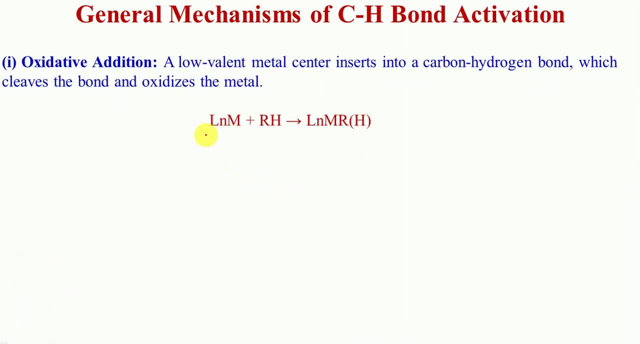 The first one is oxidative addition. The example is in front of you. I have also discussed that. as I know that I have metal, the oxidation rate of metal. first assume it is zero. Okay, Along with this here I have this RH group. I have to coordinate it. 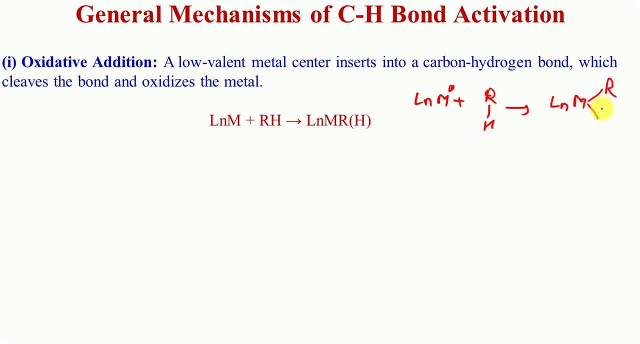 So what will be associated with LN, M and M, this alkyl group and this H, and oxidation rate will be increased by two units. Okay, So in this way we are getting an oxidatively added product in which the cleavage of the CH bond is taking place. 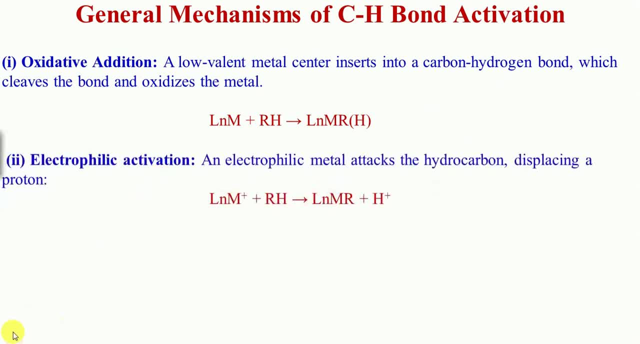 Next, the second one is electrophilic activation, As I told you earlier, which will be the electrophilic centers which are electron deficient. So you can see, here metal is in its positive oxidation state. Okay, So when the metal is in its positive oxidation state here: 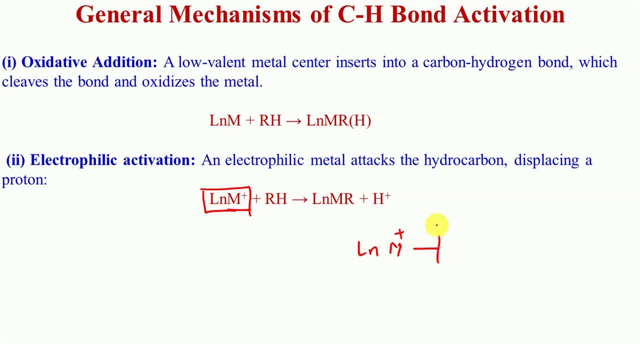 it will try to. it will try to interact with the sigma bond of this carbon-hydrogen bond. Okay, So, to complete its electron count what it will do: it will try to withdraw or try to form this sigma bond complex. 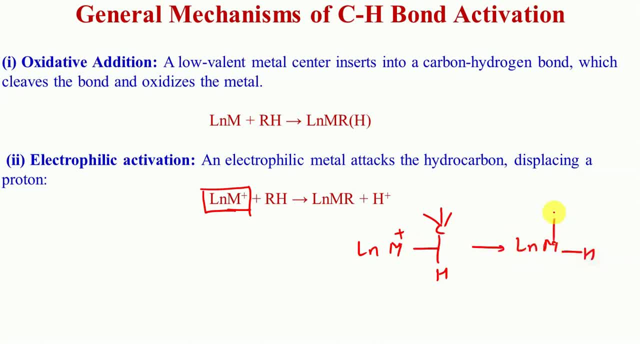 And after that what we will get? Finally, there will be addition of this alkyl substituent and hydrogen atom to the metal center. And in the last step, what happens? metal because electron is deficient already. so the electron will pull the metal from this bond and from here H as H positive. 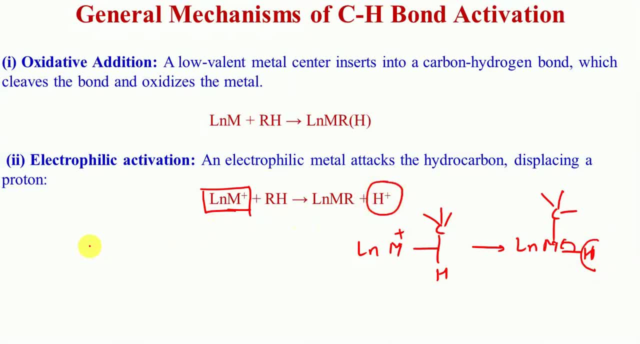 will be released, And this example is very common, very simple, which you have read. For example, if I talk about the functionalization and cleavage of the H bond of the benzene in the presence of FeCl3, as we study in Friedel-Craft, alkylation reactions, 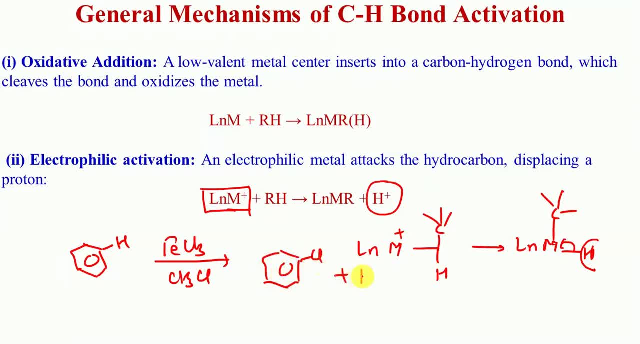 what happens? we get chlorobenzene here and along with it, HCl is released. So this is H positive which is being released here And here. no doubt metal is not positively charged, but metal is still electron deficient. 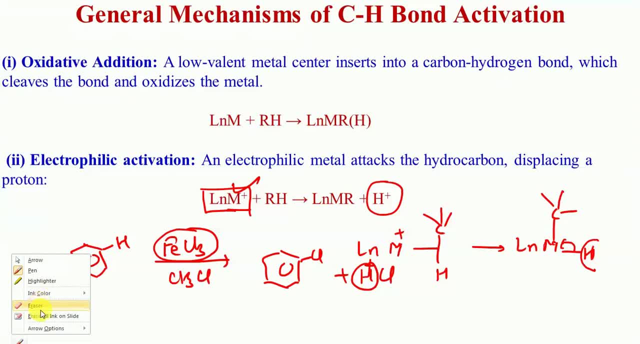 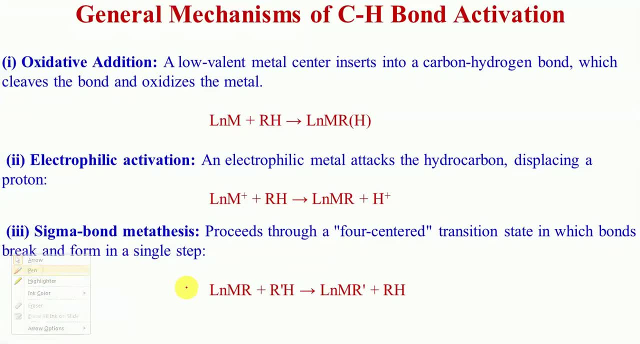 similar to this M positive part. So these were the first two mechanisms. The third one is sigma bond metathesis. So in this case there is formation of a four-membered transition state, For example. this is the complex. 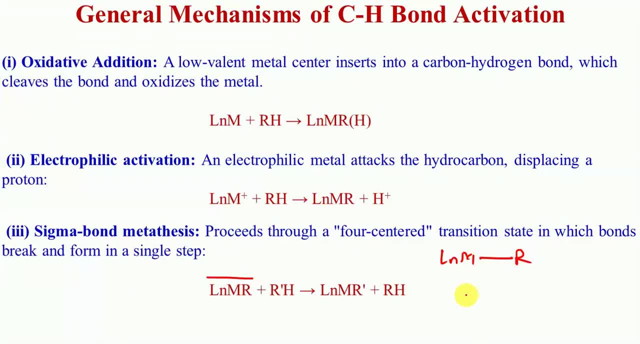 This is the complex. I have written it in this form. What will interact with it? It will interact with R-H. So this is how the interaction will show This: H will start making R bonds and will start making bonds with R-M. 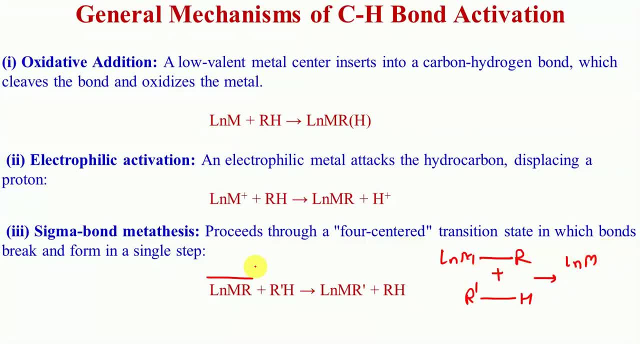 Means there is simultaneous formation of new bonds and cleavage of new bonds. So this is the process of old bond in single step. That's why it is also known as concerted type reactions. So four-centered transition state is formed, So this bond will start forming. 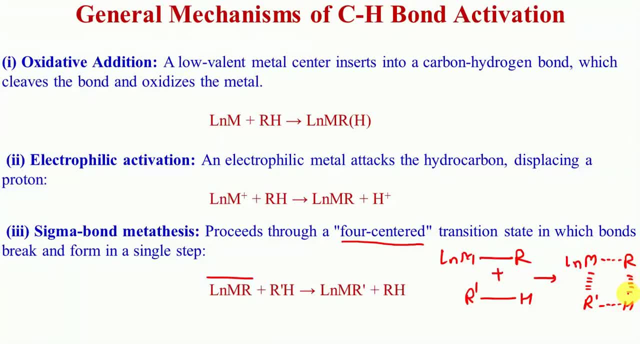 This bond will start breaking. This bond will also start breaking and this bond will start forming And in the final stage, what we will get? LMMR will form and R-H will form Means. if you had a methyl group with metal here. 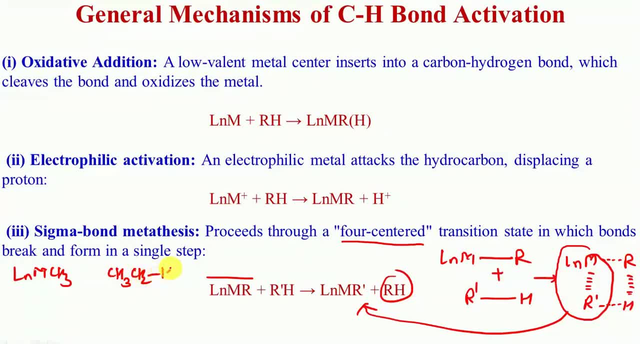 and this group- it was from ethane- then the final product we will get is LNM ethyl group and the formation of methane will take place Due to the loss of this methyl group. methane will form with this H and ethyl group will coordinate with metal. 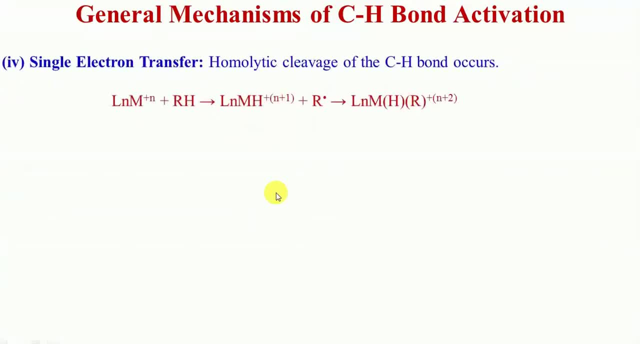 So these were the three mechanisms. The fourth one is single electron transfer. We can explain this process in two stages. The first one is, for example, we have this LNM plus N. It is reacting with R-H. This R-H undergoes homolytic cleavage and will form R-radical and H-radical. 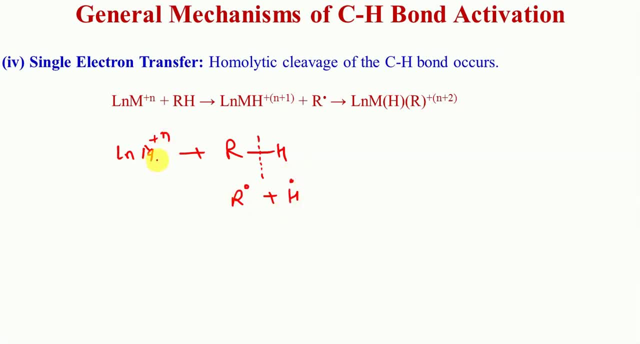 So in the first stage this M will lose one electron to H, and when H gains one electron, then H will become radical. In the second step it will lose one more electron to this R-radical and this R will become negative. 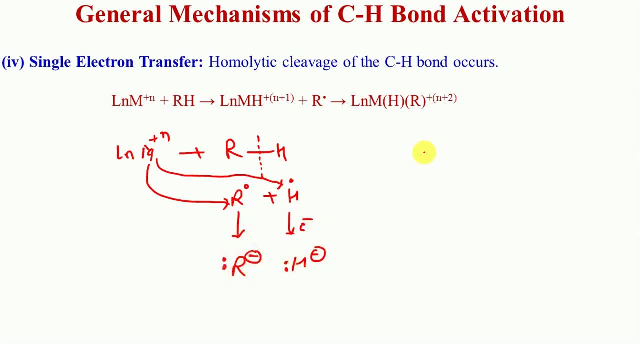 Now these two have one pair of electrons. They will be coordinating with metal to form a complex in this way. and here is the oxidation state. If it was initial plus N, then it will be N plus 2. By two units the oxidation state will increase. 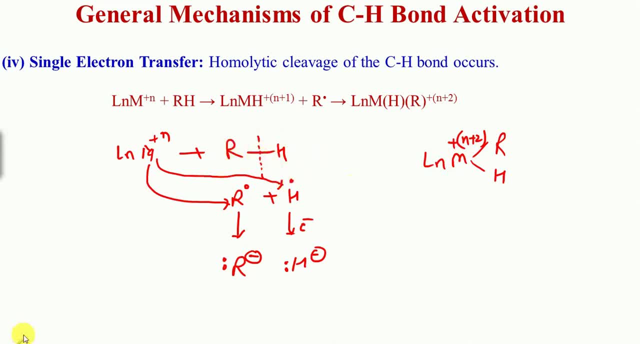 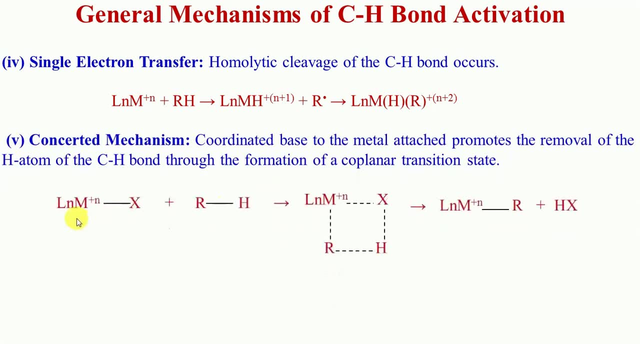 So this is one more hypothesis. It is being said that the cleavage of R and H bond will happen homolytically. The fifth step is concerted mechanism. So in this way, what happens? We need some base in this case. 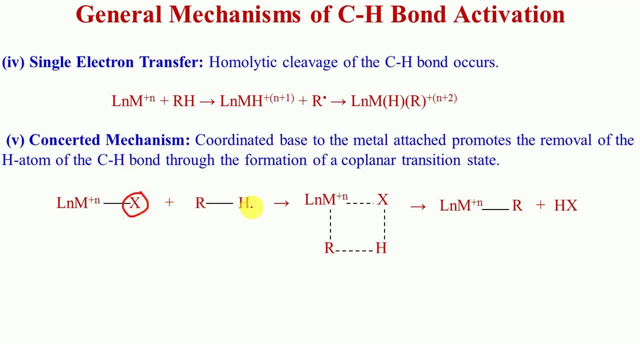 We need a base, A base that interacts with the H associated with alkyl group. So we need a base that interacts with the H associated with alkyl group. We need a base that interacts with the H associated with alkyl group. So we need a base that interacts with the H associated with alkyl group. 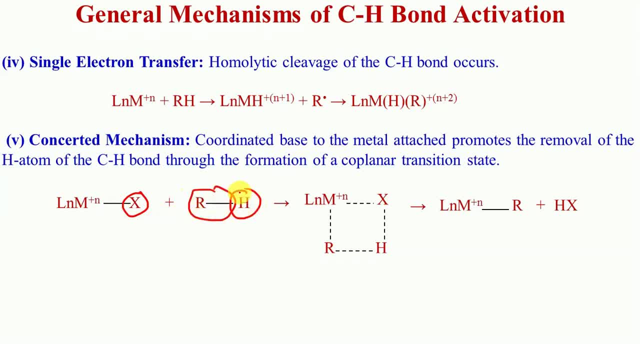 And try to make H as H-positive Means R will become negative and H will become positive. So this H-positive, this base, it can be assumed that it is NH2.. So NH2 will be released in the form of ammonia by mixing it with hydrogen. 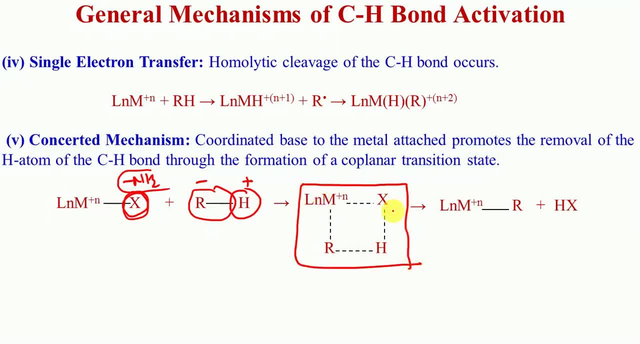 In this way, this will also make a four-membered transition state. here There will be interactions. So if this X is NH2, we will get NH3.. If this X is OH, we will get water as byproducts. And this R group coordinates with R metal. 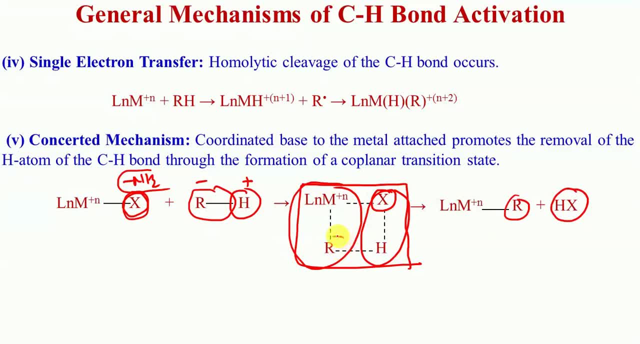 And this R group coordinates with R metal. So what is happening here? We are cleaving this RH bond. The cleavage of RH bond is happening in this case, And who is mediating it? Again, the metal center here is electron deficient. 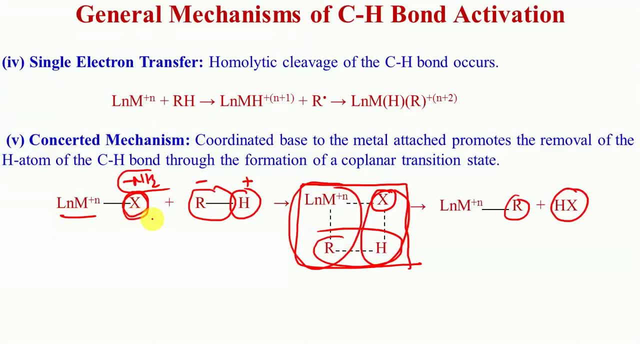 But with that deficient center we have one such ligand which is acting as base Means. metal should have a coordinated base attached to the metal which promotes the removal of hydrogen H as H-positive, Which promotes the removal of hydrogen as H-positive. 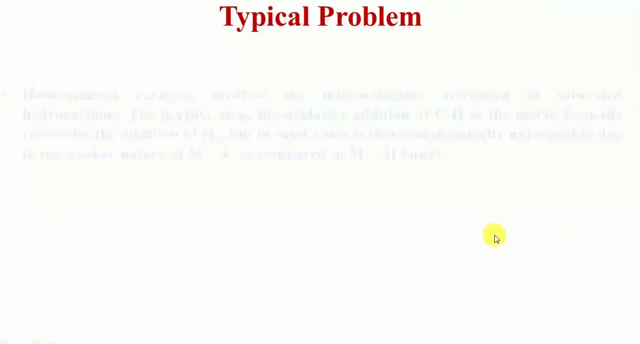 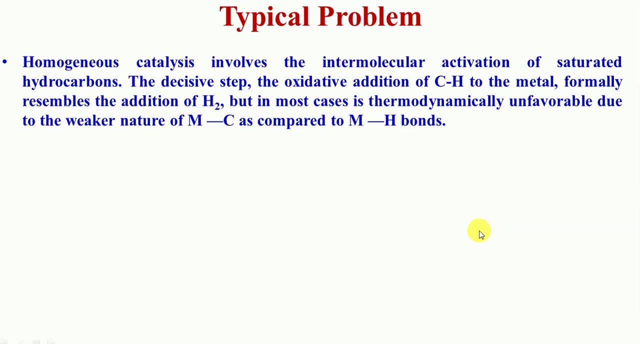 Now there is one big issue. We have also done oxidative addition of hydrogen in many organic metallic compounds, But the oxidative addition of hydrogen is quite different from that of the oxidative addition of CH bonds. And what is the reason for that? So see here. 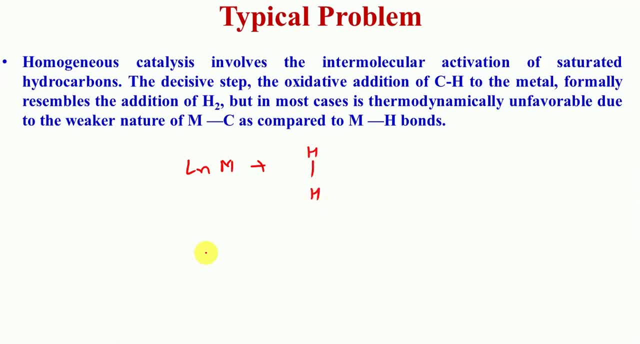 I am explaining it in this way. So we have this complex: In the first case we have H-H bond And in the second case we have CH bond which will coordinate And the product which we will get will be LmH. 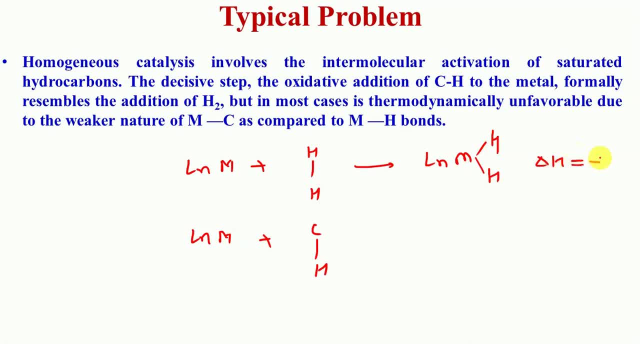 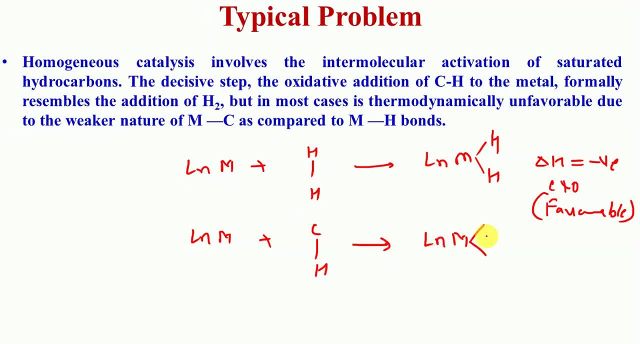 So it will happen easily. So it will happen easily. So in this case the bond which will be made with metal is carbon. The bond of hydrogen will coordinate in this way, But in this case the delta H is positive. 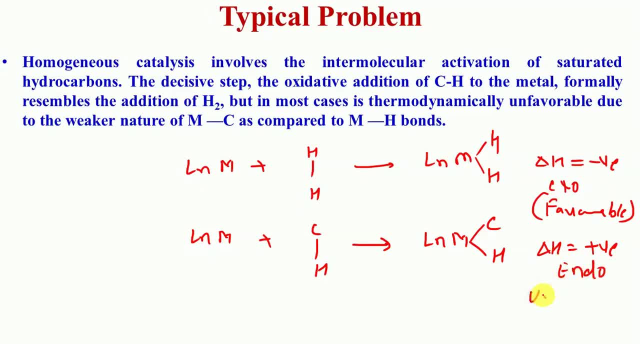 Means. the process is endothermic, So it is thermodynamically unfavorable. So this is the main difference between the oxidative addition of hydrogen and CH bond into metallic compounds. So it is very easy to oxidatively add Or cleave this hydrogen-hydrogen bond, as compared to cleave, the cleavage of this carbon-hydrogen bond. 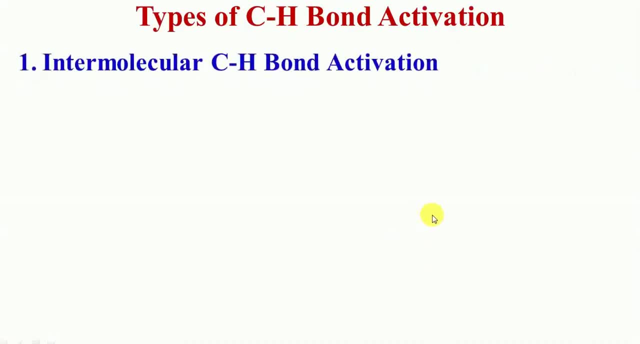 Now there are two types of CH bond activations. The first one is intermolecular CH bond activation And the second one is intramolecular CH bond activation. So we will discuss these two in detail, Which one is intramolecular and which one is intramolecular. 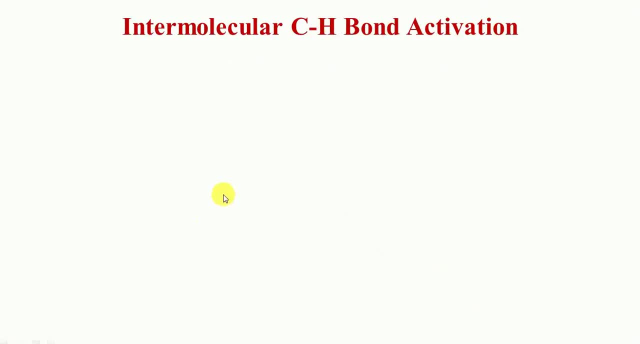 So first of all we will talk about intermolecular oxidation. So what happens in intramolecular CH bond activation? The complex we have is this: It will react with some hydrocarbon which we are adding from outside. So finally we will get L, N, M, R and H. 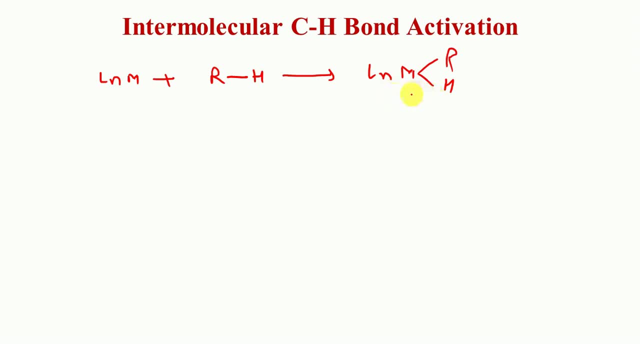 So this type of CH bond activation is called intermolecular CH bond activation, In which complex is reacting with some hydrocarbon. I am explaining you some examples of this here. So this is cyclopentadienyl ligand. In this there are methyl substituents on every position. 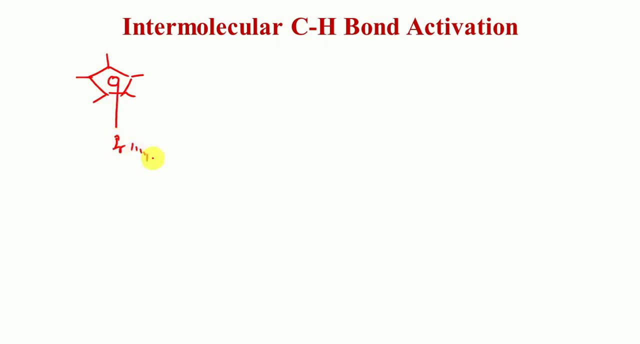 This is eta-5.. With this is iridium. With iridium, we have one hydrogen here, One hydrogen at this position And one trimethylphosphine ligand. Okay, So when it reacts with Neopentane. 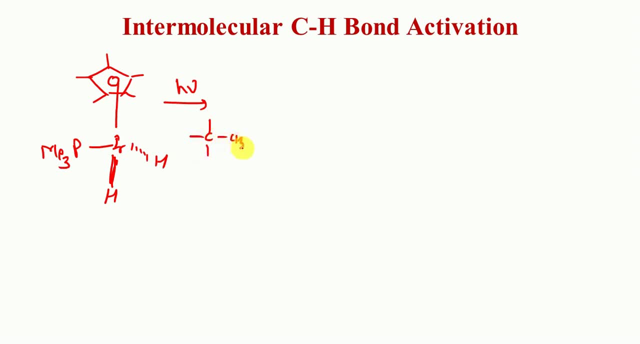 Now, what is neopentane? Neopentane is this group: Here CS3.. Here CS3.. Here also CS3. And here also CS3.. So, in this case, what we will get This is cyclopentadienyl. 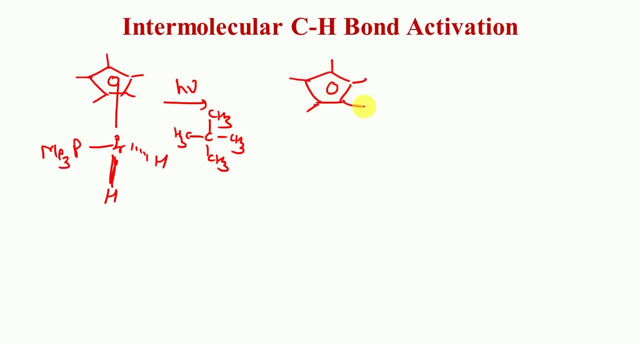 It is methyl substitute. There are methyl substituents on every position. We have iridium With iridium, it will come here With H, And what will it coordinate with H? We have CH2.. CH3.. CH3.. 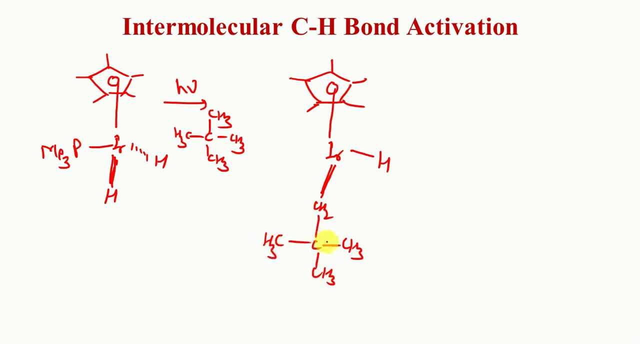 CH4., CH5., CH6., CH7., CH8., CH9., CH10., CH11., CH12., CH13., CH14., CH15., CH16., CH17., CH19., CH19., CH21.. 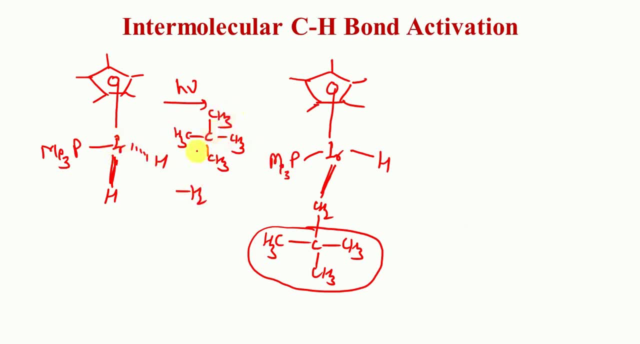 CH22., CH23., CH24.. CH25., CH26., CH27., CH27., CH28., CH28., CH29., CH30., CH30., CH30. At first we have oxidative addition with metal. then these two H are removed from here as H2. 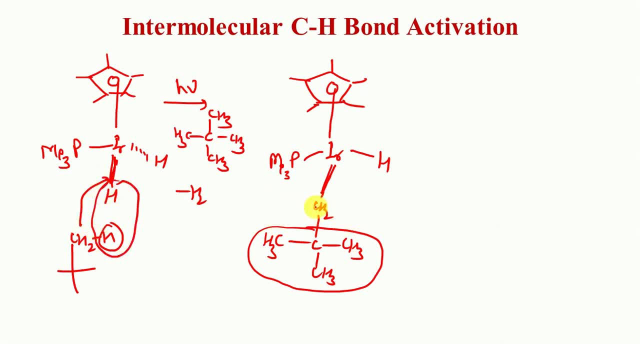 and this carbon atom will coordinate here. So in this way we will have this neopentyl compound attached, neopentyl group attached to this iridium complex. So first step is oxidative addition of neopentyl or neopanthane. 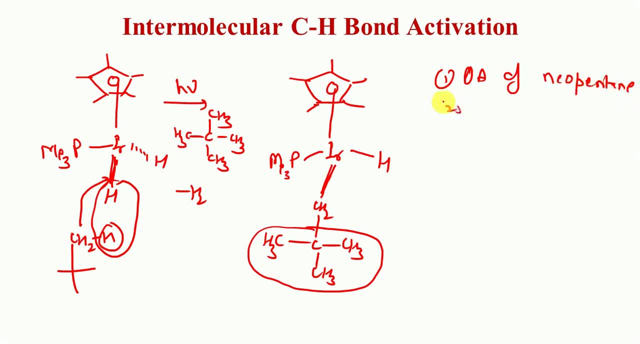 you can say: And then there was reductive elimination of H2, so we will get this as a reduction of H2, also called CDYeah, final product. This was the one example. There is one more example. We have again a complex of. 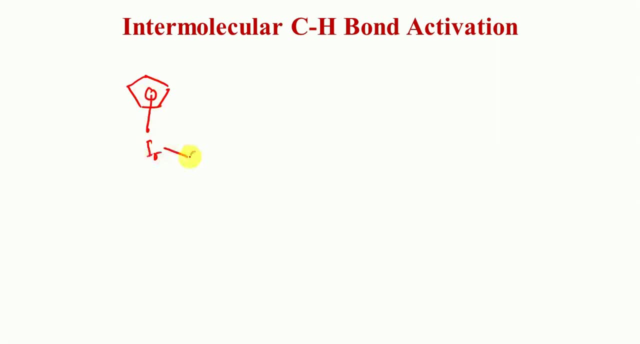 iridium or iridium ke sath hai, yaha pe 2 carbonyl groups. There are 2 CO groups. Jab ye react karega with C6F12.. Now what is this C6F12?? This is fluorosubstituted cyclohexane In the presence. 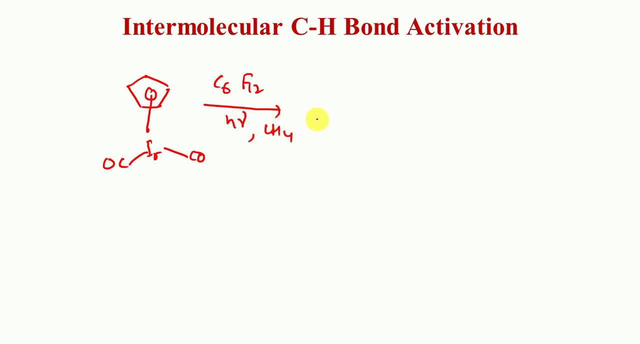 of light or methane, what we will get, Minus CO 1, carbon monoxide, ligand yaha, se remove ho jayega And what we will get. We will get iridium Yaha, pe H. agaya 1 H kaunsa. Methyl group ka: 1 H yaha. 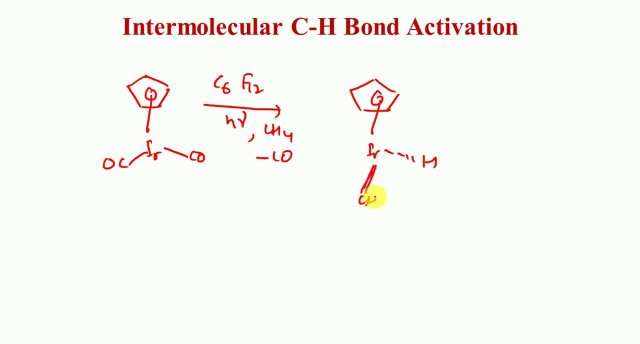 pe agaya 1 methyl iske sath coordinate kar jayega. This is methyl group Aur 1 CO group, jo pehle hi yaha pe bada ho hai, To 1 CO remove ho jayega Aur uski jaga pe 2 aur positions. 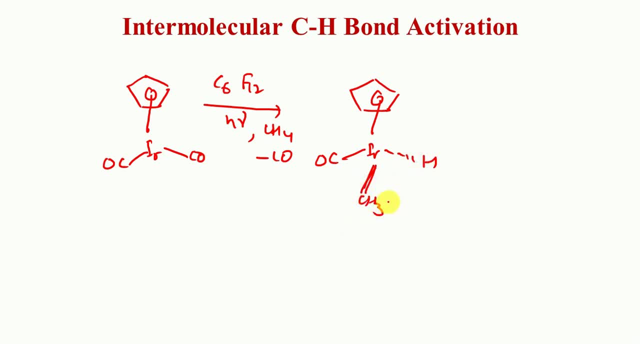 occupy ho jayega 1 hydrogen aur 1 methyl group. usko Jaha kahan se ayega Methane se Aur iss reaction mein. we need 10 bar of atmospheric pressure. This was the second example. In third case we have this ethene phosphine jismein 2 cyclohexyl. 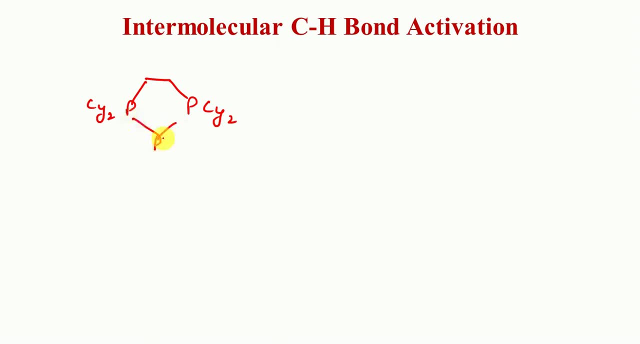 substituents hai Aur ye compound bana raha hai, platinum ke sath, Platinum ke sath hai, ek taraf ko H aur ek taraf ko hai group jo abhi humne peechhe bada. It is 1 H and 1 H2O. 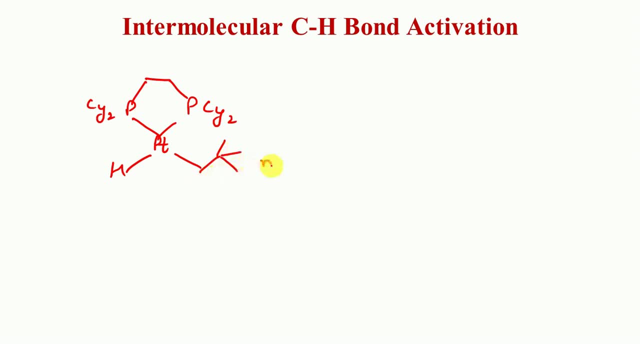 This is neopentile group. This is neopentile group At 45 degree centigrade temperature. yaha se neopentane remove, ho jata hai means there is loss of this neopentane. Neopentane. 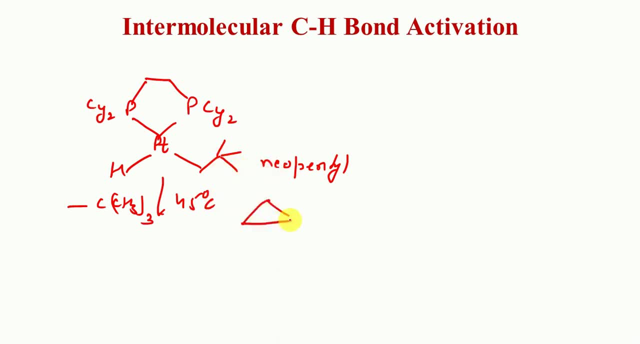 remove ho jayega aur isme addition. kiske karenge. We will add cyclopropane derivative To ye derivative attached ho jayega aur humar par ataj hai. You can get the addition value. Keep desciptor, same for you. Keep desciptor, same on it. Keep desciptor, same on it, Keep desciptor. 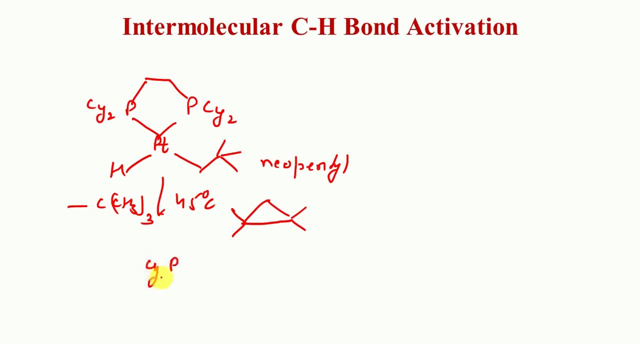 complex will be p, then we have platinum and finally one H will be here and one group, which we are adding molecule will be formed like this: so this CH bond, this CH bond is activated. so this was intermolecular CH bond activation, in which 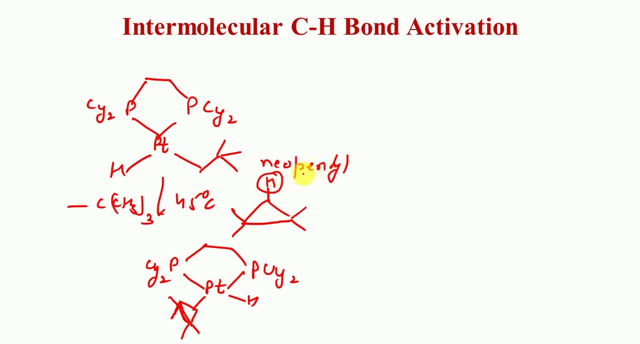 we are adding reagent from outside and that reactant may be Hydrocarbon and Aereans. its CH bond is activating. The other category comes to us, that is intramolecular CH bond activation. so in the case of intramolecular, one topic you have already studied and that is 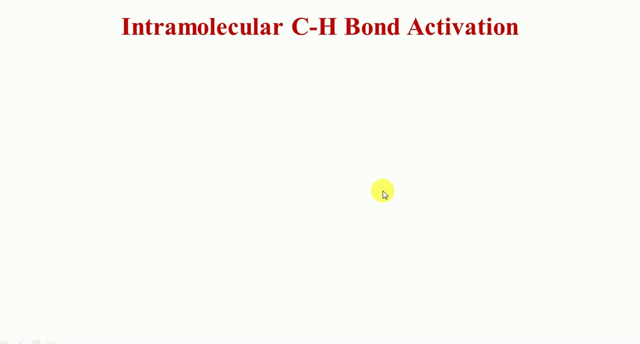 called Orthometallation or Cycl, exponentially o, photo methyLation. we have studied Orthometallation, our Cyclometallation. so this is the example of Orthometallation. This is IR. we have Cl. then here we have 3 triphenylphosphine substituents. 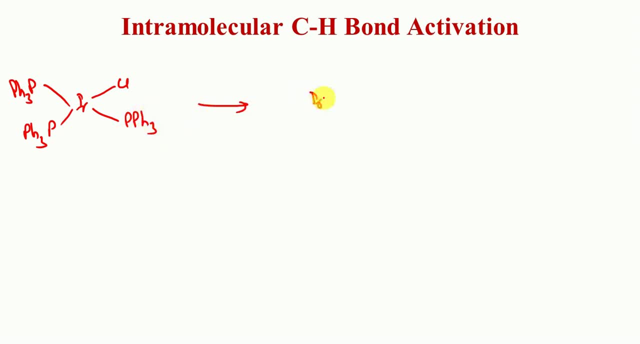 What will happen in this? This is 16 electron compound iridium. compound iridium oxidation status is plus 1.. So with iridium, here is 1 Cl. Here, among the 3 phenyl substituents, 1 oxidative addition shows here with iridium. 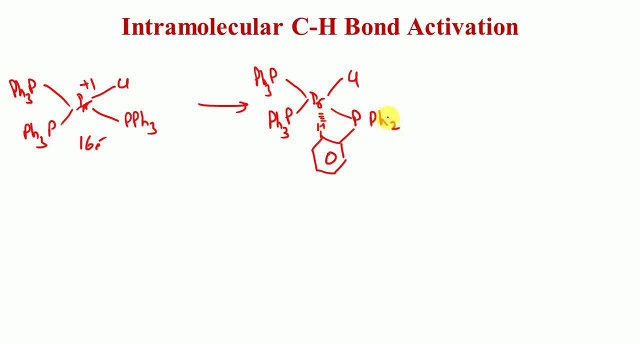 So here H will be there. With this H, iridium-agostic hydrogen interaction will show, And after that this compound will be oxidatively added here, And what we will get? We will get a 6-coordinated complex. 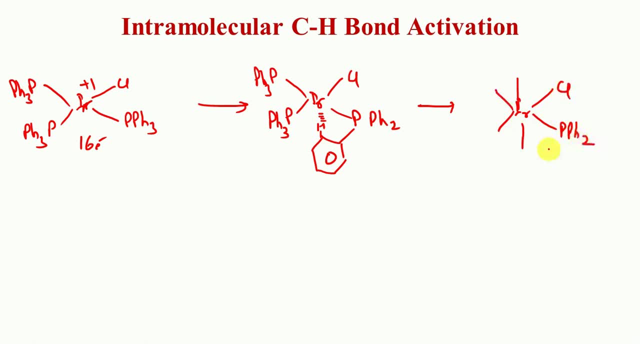 Here is Cl, here is PPH2.. Here we have a benzene ring attached to it. In this way, 1 H came, which came out of this position. Benzene ring's CH bond was there, It was cleaved, it was activated. 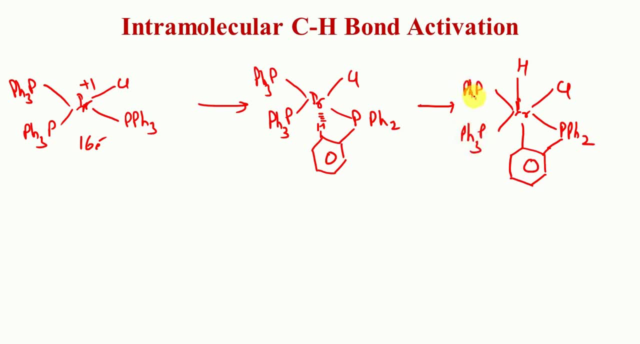 Rest of the substituents as it is written here. So what is there in this Oxidative addition, is happening in this? But we are not activated. We are not adding any reagent, The one whose CH bond has to be activated. it is present in the group, present in the same compound.